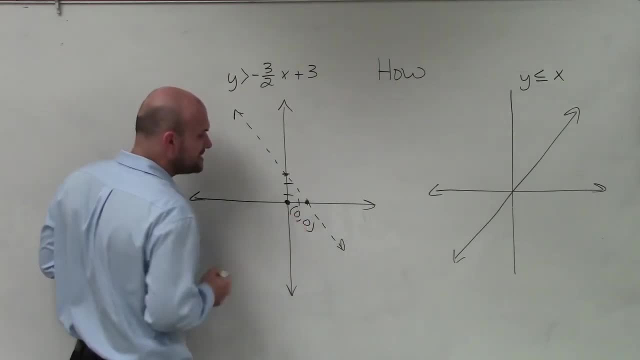 through that point. Now. the reason why is so helpful is we'll, first of all, because the operations are going to be very simple Compared, because any time you're adding to zero or multiplying by zero, it's a pretty easy operation. Now, 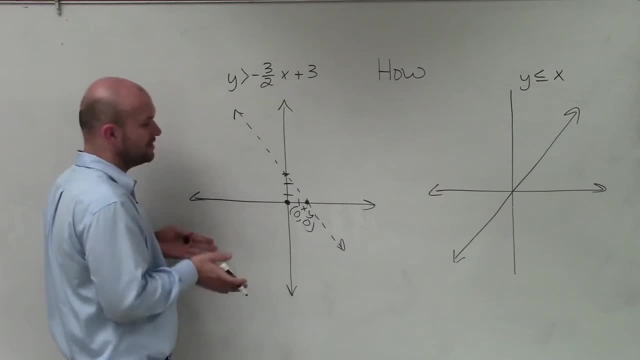 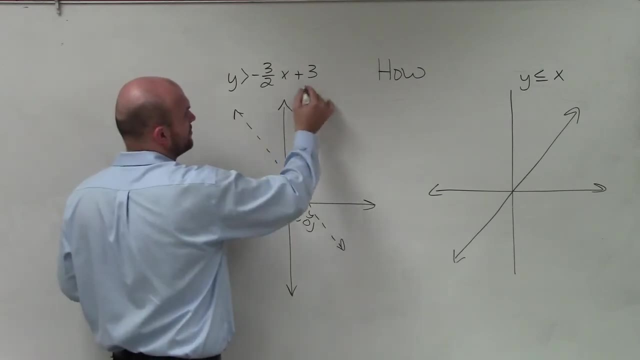 remember the point has an x and a y coordinate. So what we're going to do is we're going to plug zero in for x and zero in for y in our inequality And we're going to see: does this make the inequality true or not? So I plug in: zero is greater than negative. 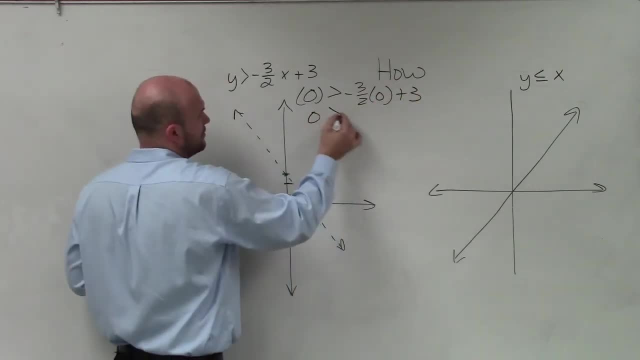 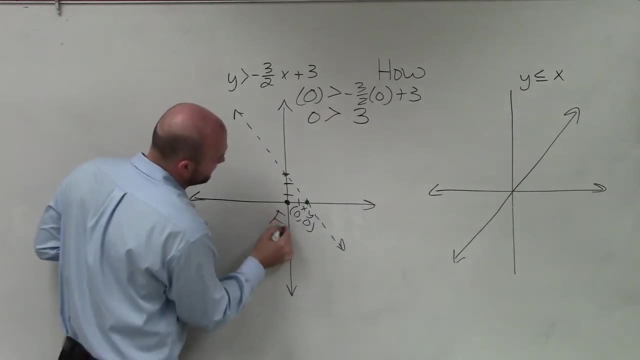 three halves times zero plus three. Zero is greater than negative. three halves times two than negative. 3 halves times 0, obviously is 0, plus 3 is just going to be 3.. 0 greater than 3, that is false. So what that means is, if one point below the line is false, that 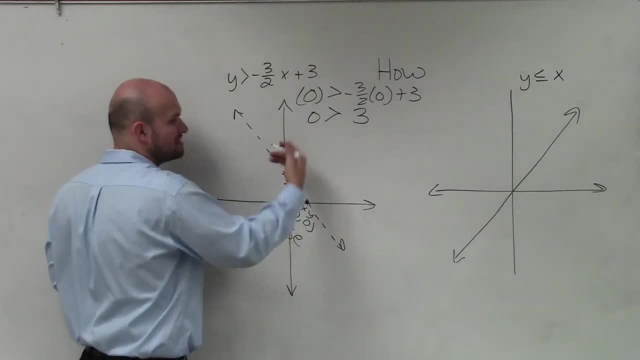 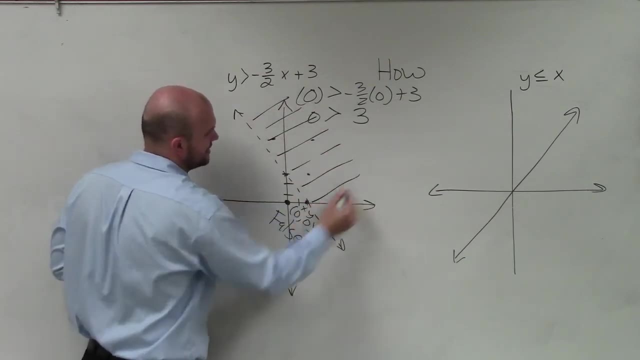 means all points below the line are false and that means all points above are true. That means that's true, that's true, that's true. So rather than plotting all those points, we just kind of do some nice little shading here Now to kind of show you also why the 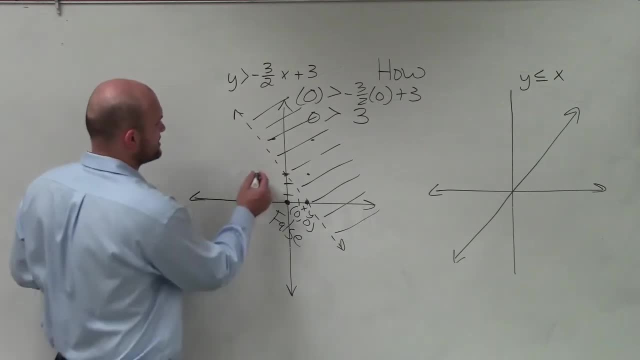 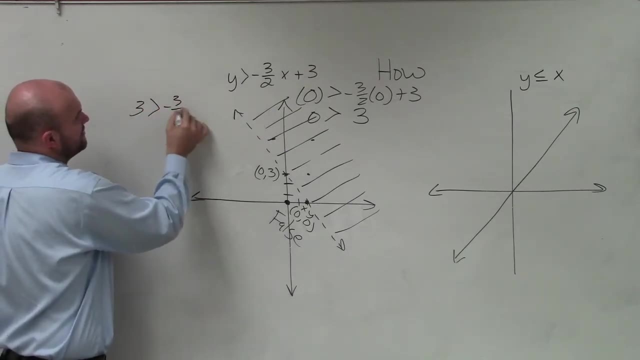 points on the line are false, why we're doing a dash. let's pick another point, 0 comma 3, real quick and show you why that doesn't work. because it is false. So I have: 3 is greater than negative, 3 halves times 0 plus 3.. Again, that's 0.. 3 is greater than 3.. Well, 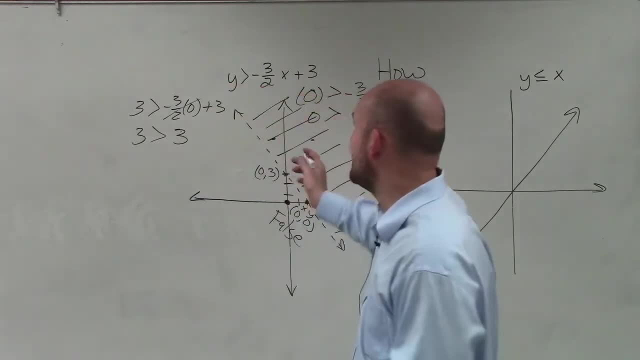 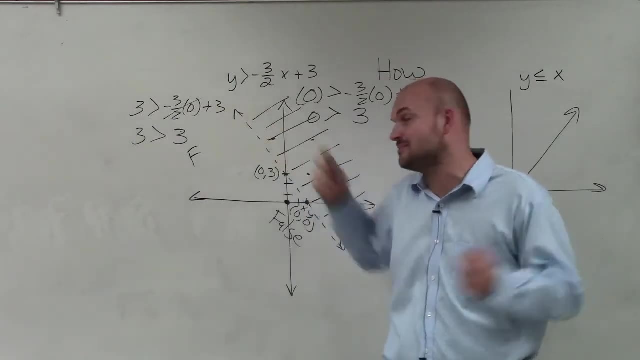 3 is never greater than 3, right 3 is equal to 3, so that's why that is false and it's dashed line. But I think it's much easier just to look at the inequality symbol. Less than or greater than. it's always going to be false. Now we have a dilemma over here. 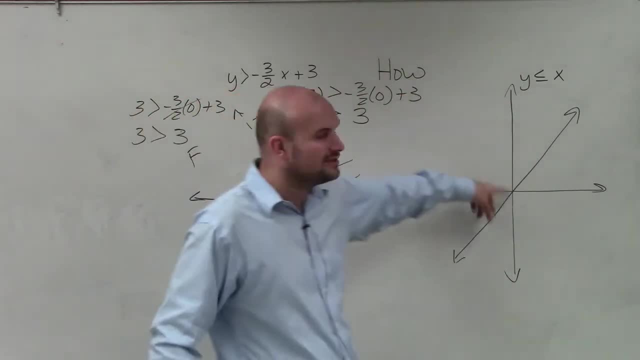 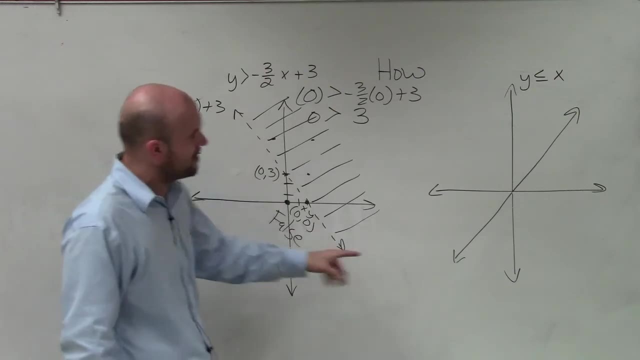 Because here I always say 0, 0, but now 0, 0 lies on the line. So if we use 0, 0, it's like me testing this point again. We already know what the line is. This one's not a part. 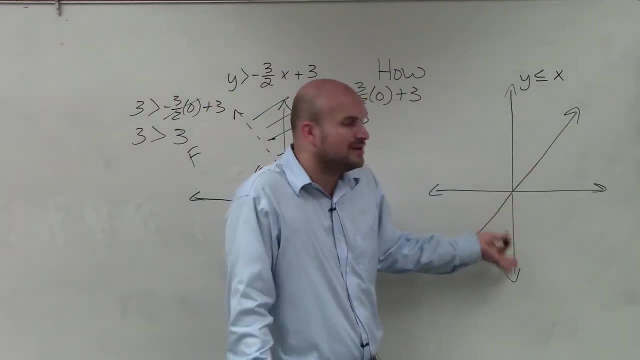 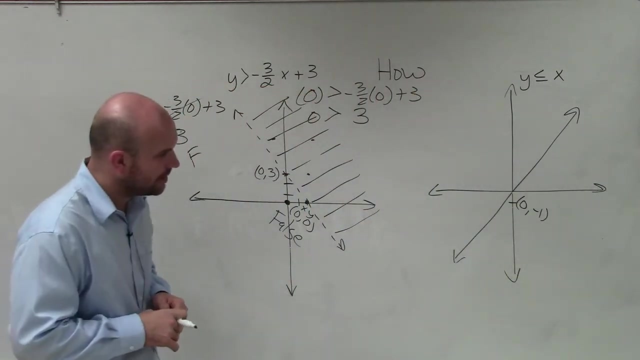 of the solution. The points here are all a part of the solution, So there's no point in testing 0, 0.. What I'm going to want to test here is a point above or below, So let's go ahead and choose this point: 0 comma negative 1.. So when testing 0 comma negative 1, again,